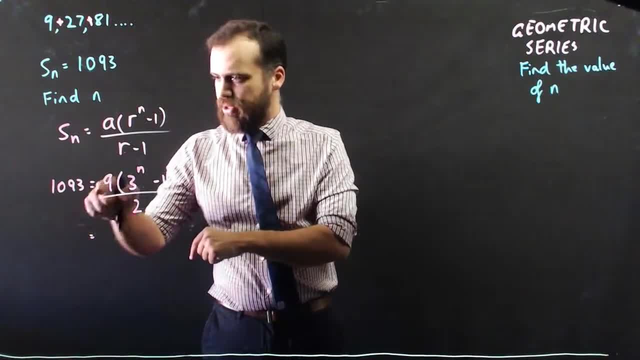 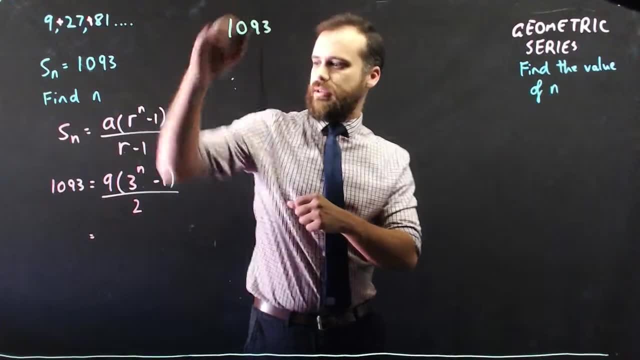 Multiply everything by 2.. That'll get rid of the 2 from there. Divide everything by the 9. That'll get rid of the 9 from there. So the next line's going to be something like 1093 times it by 2, divided by 9.. 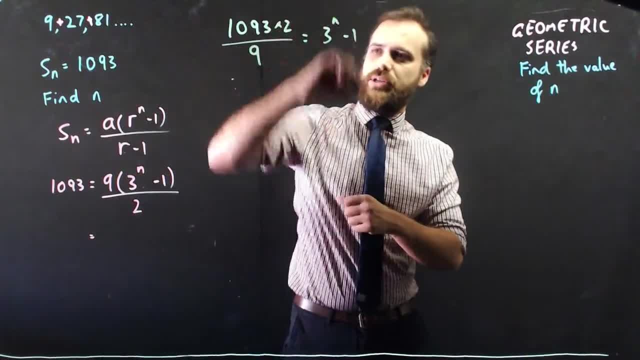 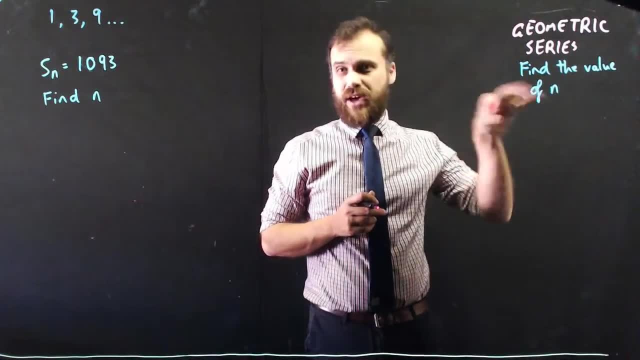 9.. So that's going to be 3n minus 1.. Calculator: All right. so geometric series. again, This time we're going to find the value of n, So it's a question something like: here's our geometric sequence: 1,, 3,, 9.. 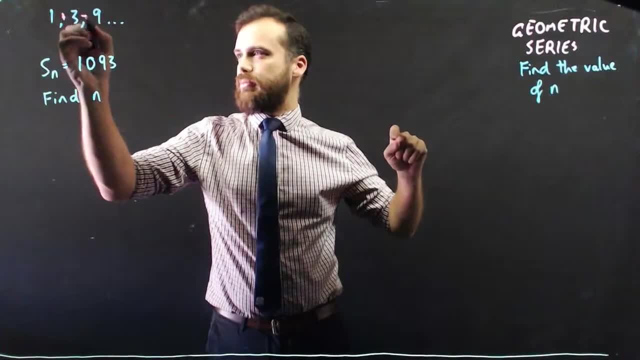 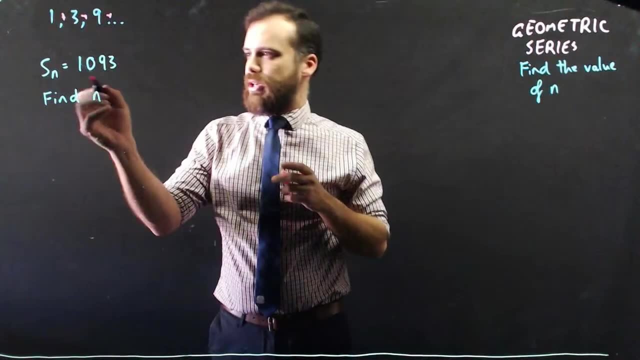 We're going to add them together: geometric series, So 1 plus 3 plus 9 plus, etc. etc. Now how many terms would we have to add together to get 1093?? So Sn, Sn. What's the n value for that? 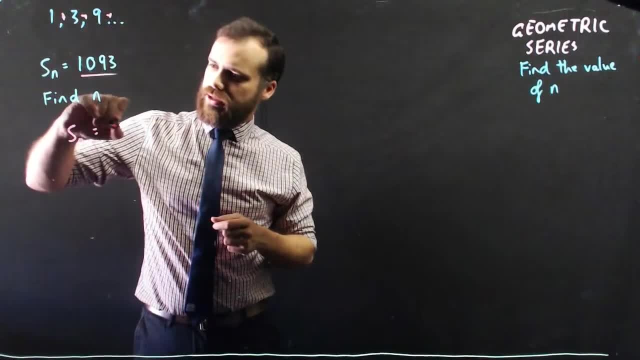 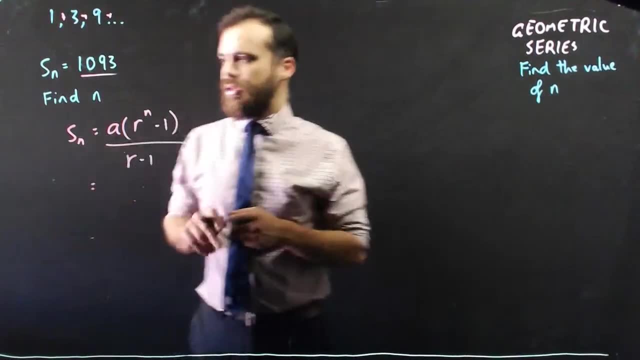 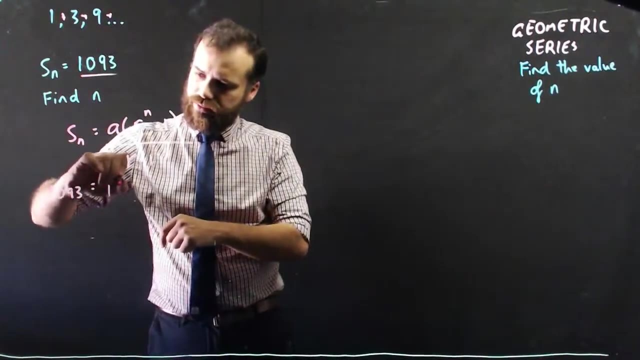 So our geometric series formula is a bracket r to the n minus 1 over r minus 1.. In this case, Sn is 1093.. The a value first term is 1.. The common ratio, 3 divided by 1, is 3.. 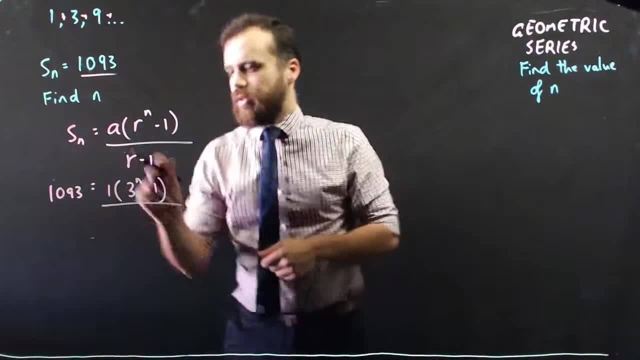 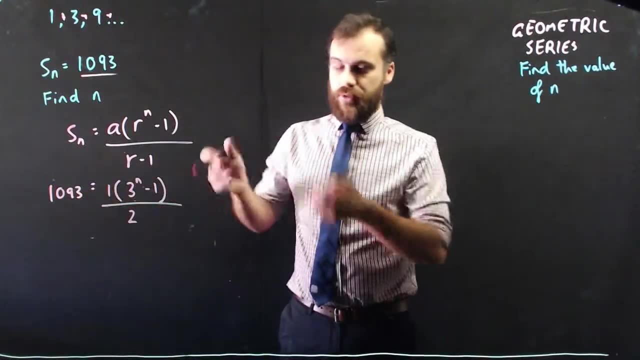 So 3 to the n minus 1 over r minus 1,, 3 minus 1,, which is 2.. Okay, So pretty much from there. we just need to rearrange this thing Now. the 2, we can multiply by the 2.. 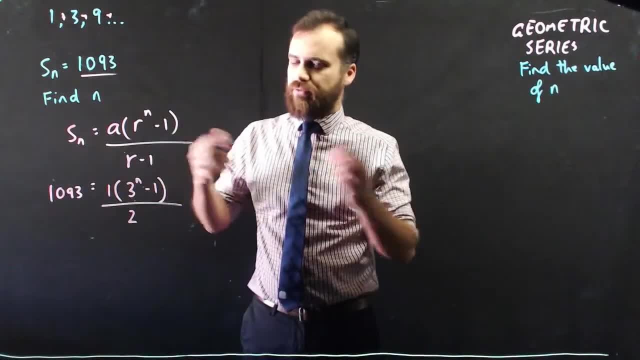 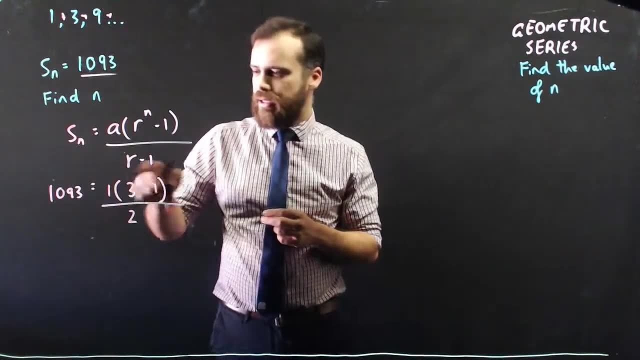 And the 1 here. if the 1 was a different number, like 5 or 7,, you might be tempted to expand the brackets and do 5 times 3n, 5 times negative 1.. What you're better off doing, though, is dividing by that number. 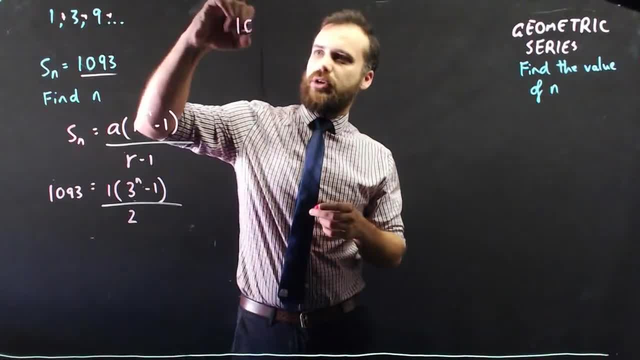 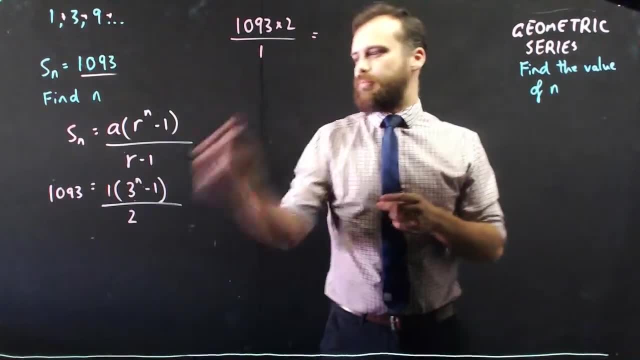 So, even though we don't need to divide by 1, I'm just going to put it in my working just so you can see what I would do, Okay, If that number wasn't 1.. So I'm multiplying by 2, I'm dividing by 1, not that that changes anything.